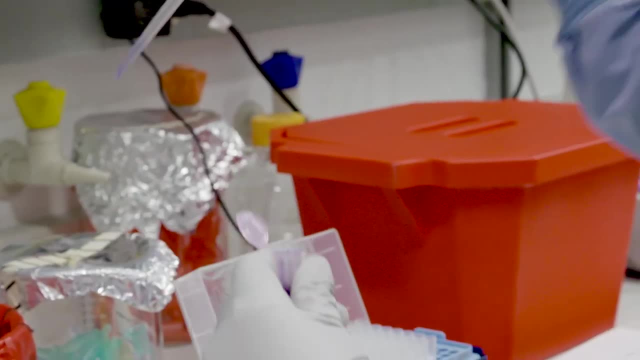 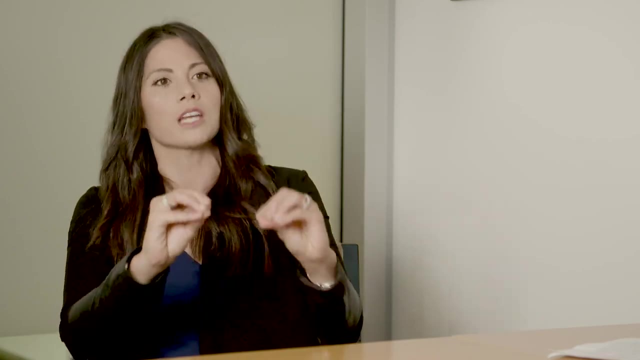 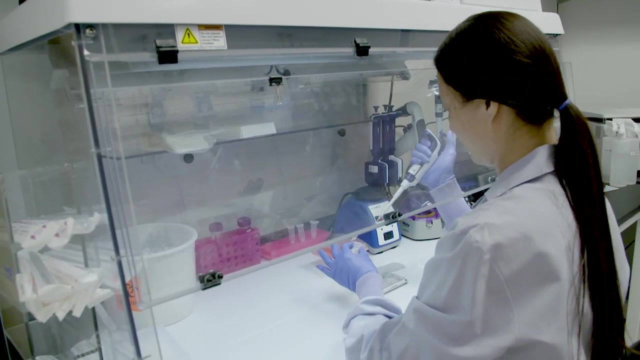 apply later to other patients coming through the door or through clinical trials, and personalized treatment tailor-made to the person having the specific variation or genetic mutation that we've now identified in their genomic sequence. The Center for Bioinformatics and Functional Genomics is really crucial to driving forward the research that we're doing in the 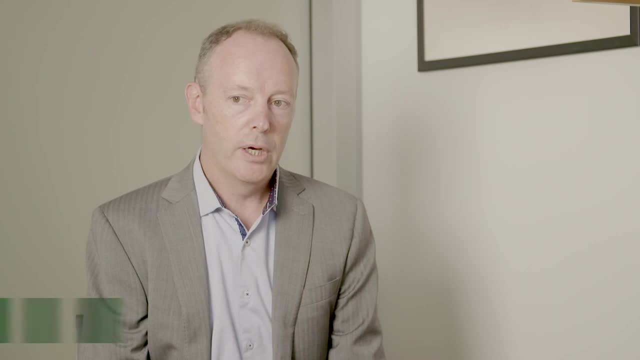 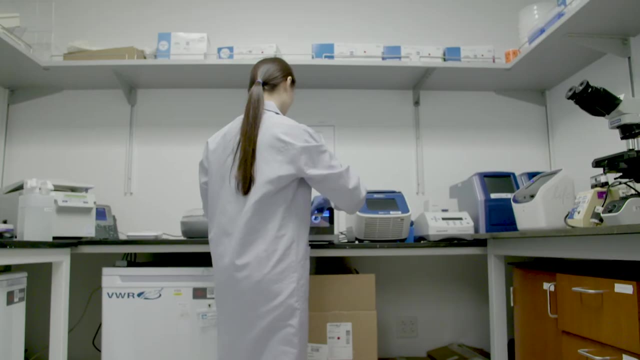 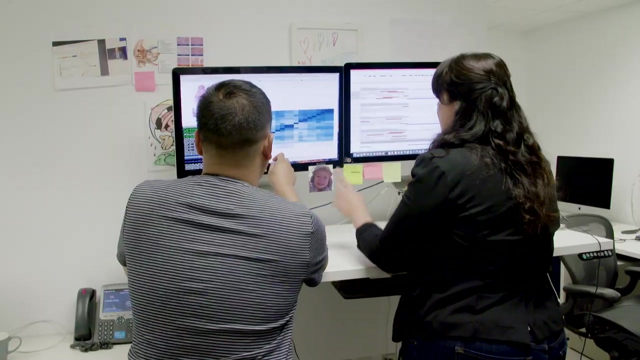 field of precision, health or personalized medicine. We regard it as a very integral part of the whole setup to help us achieve our aims in that area. The group will be generating multi-omic data, will be interpreting it and, very, very importantly, will be helping us implement it, so bridging that final gap. 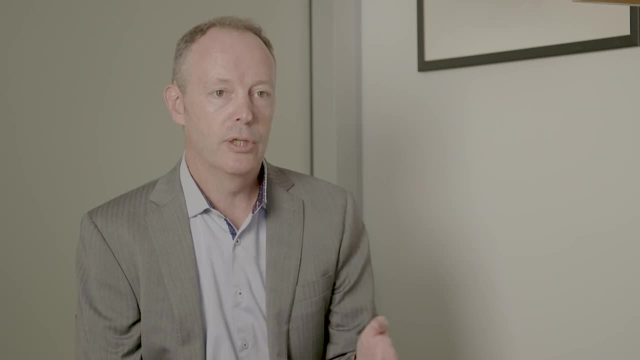 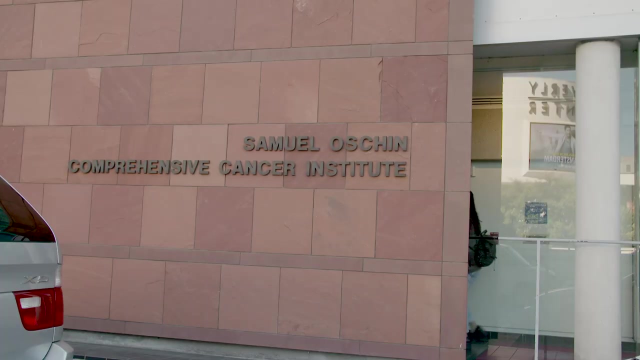 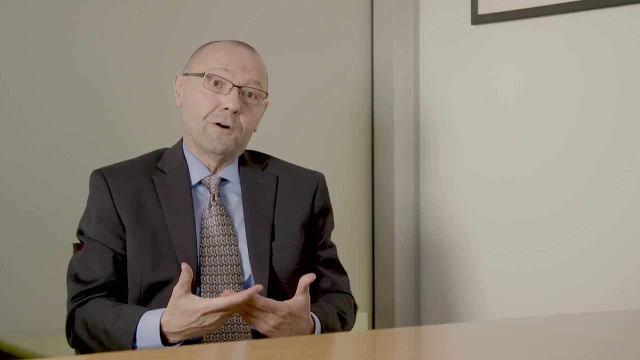 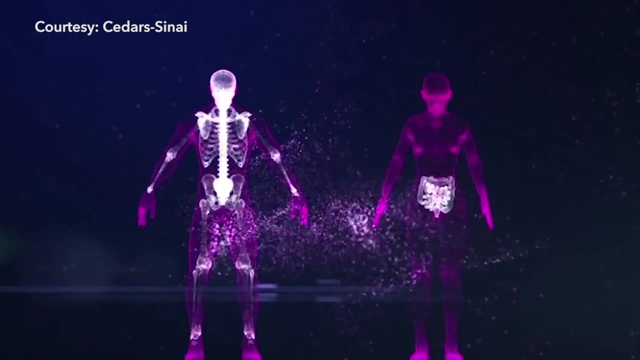 of getting this research through to clinical practice. One of the most critical ways that I think about omic technologies changing cancer medicine is really in the development of tests based on omic discoveries that can actually profile patient tumors and then, based on that profiling, develop a test that will assign patient to specific and 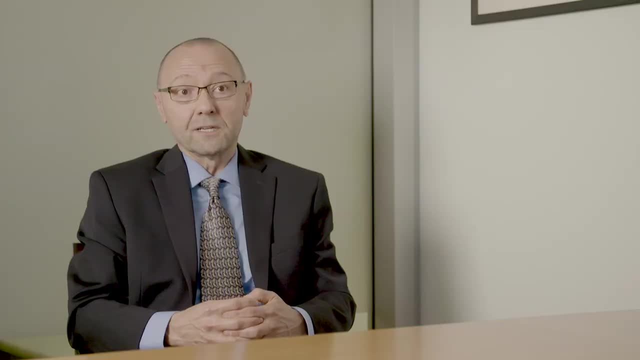 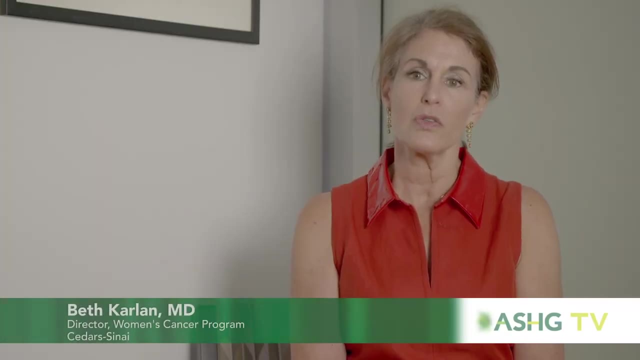 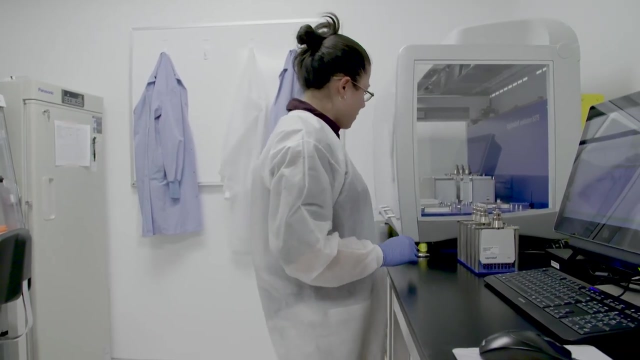 precision therapies. This whole area is a very active area of investigation in the Cedars-Sinai Cancer Center and obviously in collaboration with BFG Oncologists who's cared for many patients- women and patients with cancer. it's been a long time challenge to better. 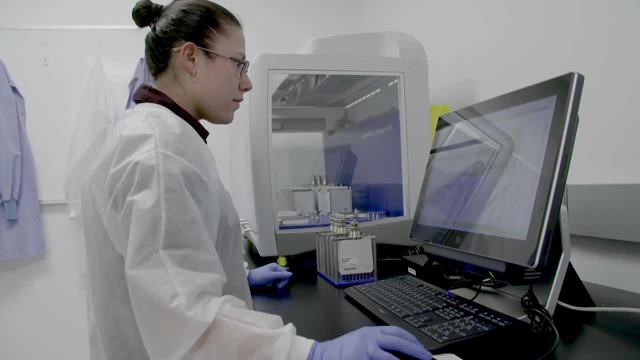 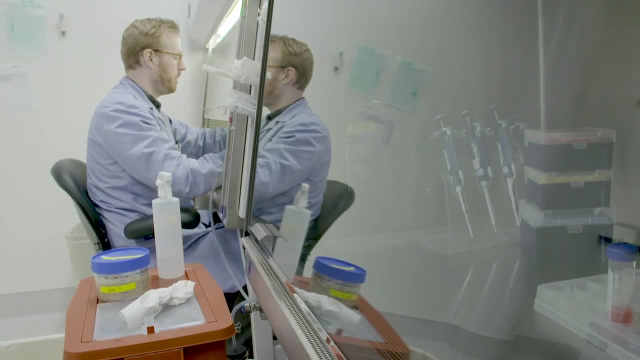 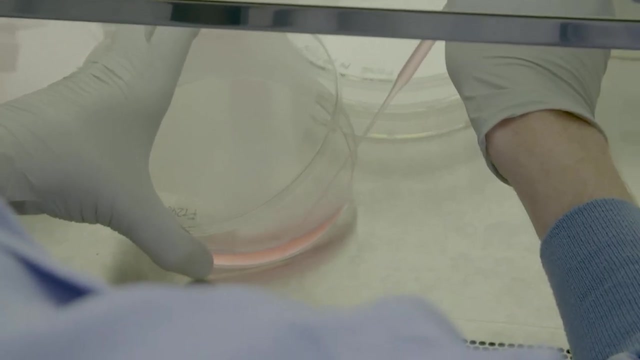 understand why some patients get cancer and others don't, why some patients survive and others don't. The collaborations and science we're doing at the Center is finally giving us some rational understanding of how to approach these diseases. I think the future will allow us to understand who's. 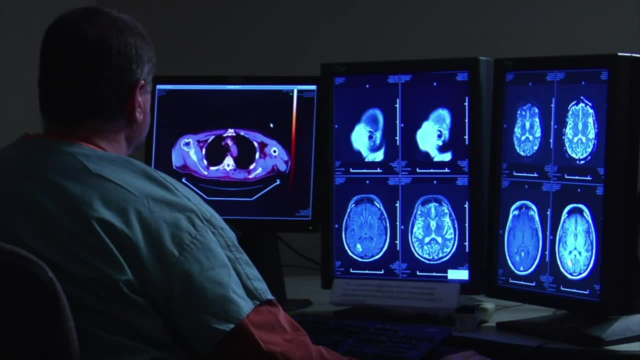 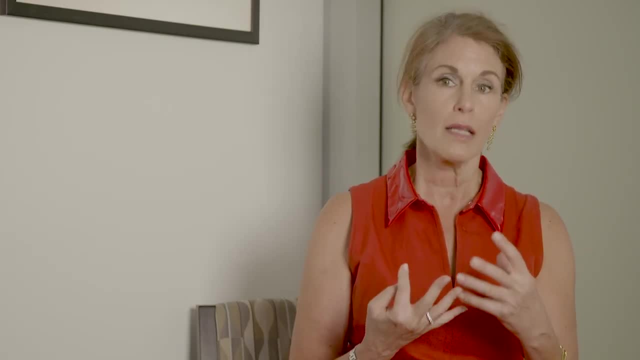 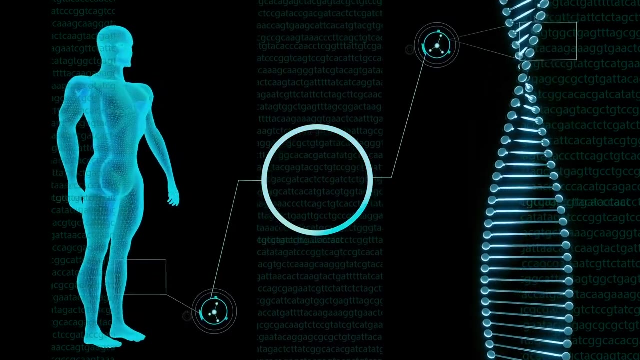 at greatest risk, why they're at greatest risk, what we can target to reduce those risks. To me, the gold ring that I want to grab is not a cure. it's really prevention. In 20 to 30 years, everyone will have their 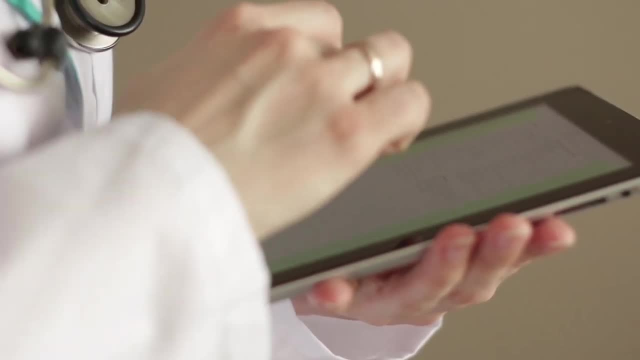 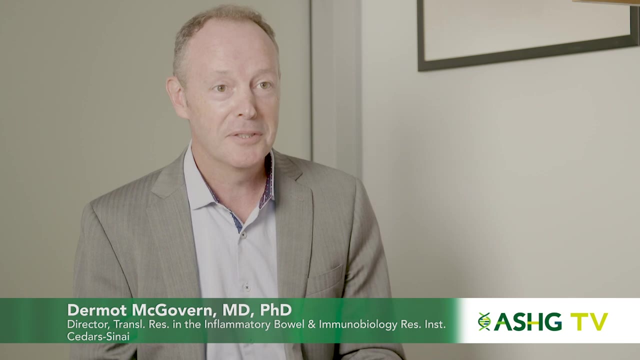 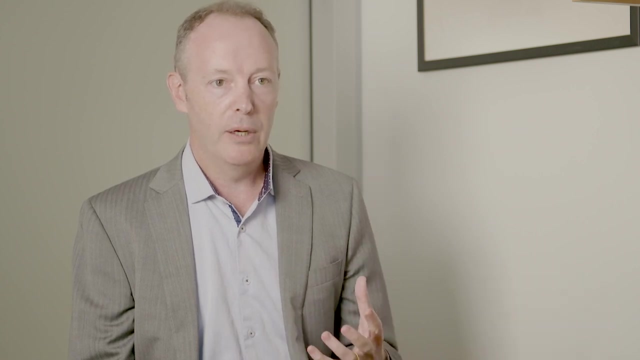 genome sequenced at birth. They'll have that data attached to electronic medical records. They'll carry it around on whatever the current edition of a iPhone is. In addition to that, they'll have proteomic data, will understand their microbiome and will understand the